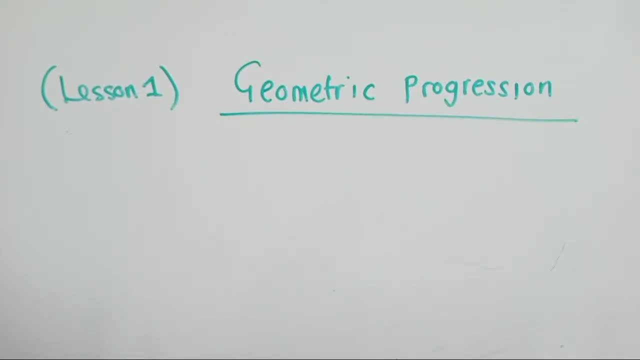 Tell your friends. you know that there's a lesson right now, So we need to do this lesson. Let me just wait a bit for people to join, Like the video, share and tell more as many people as you can so that we do the introduction of this lesson And also confirm if it's clear. Are you able to see what I'm writing or what I've written here? 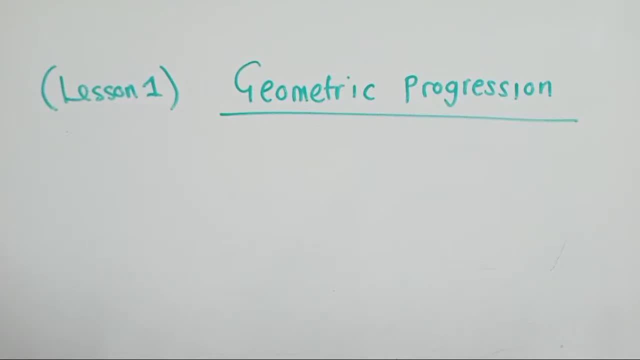 Hello hello, Hello hello. This is lesson one, So share the video. Kindly share the video. If you have a group that you are in WhatsApp group, be it Facebook, share the link so that people can join And don't forget to like. So can anybody confirm if it's clear? Is it clear? We do lesson one on GP. Is this clear? 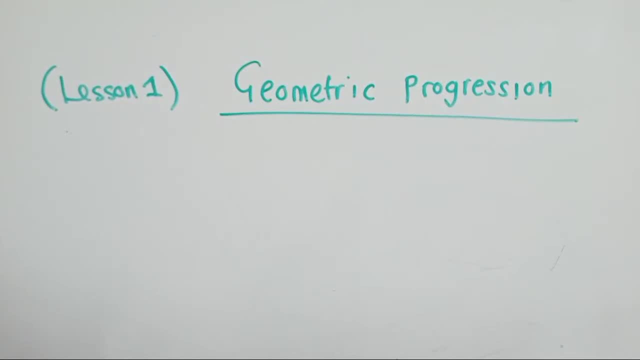 Yeah, just comment. if it's clear, We start. Okay, Susan, I can see Susan Banda is saying good evening, All right, So let me just start For those who have not yet joined. they will join us later, All right. So this is lesson one, And when it comes to this topic- geometric progression- this is a topic that 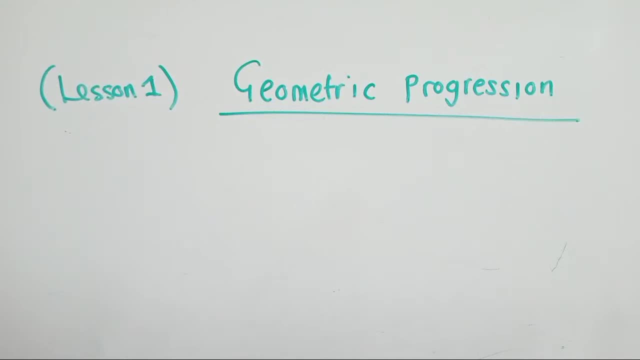 that quite number of people face difficulties on. The reason is they forget to follow simple rules. Okay, They forget to follow simple rules. So, rule number one: you must understand the terminologies. Okay, Okay, Okay, Okay, Okay Okay. 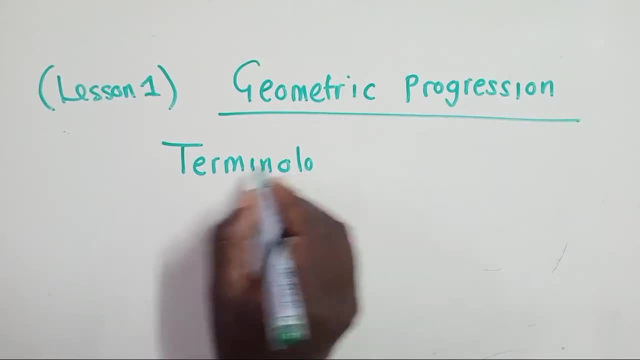 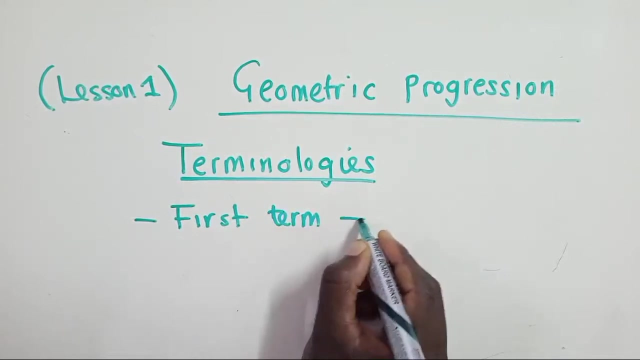 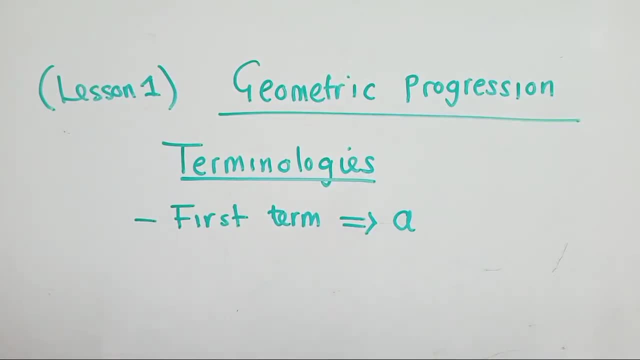 Okay, All righty. Thank you, Ellis. Okay, Okay, ppy of information today, my dear cafeteria, Yeah Yeah, is the number that is at the beginning or starting point of the sequence. okay, the next thing that we must be aware of is the common ratio: common. 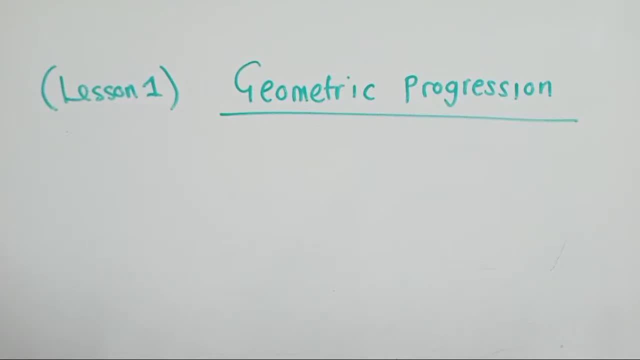 Hello hello, Hello hello. This is lesson one, So share the video. Kindly share the video. If you have a group that you are in WhatsApp group, be it Facebook, share the link so that people can join And don't forget to like. So can anybody confirm if it's clear? Is it clear? We do lesson one on GP. Is this clear? 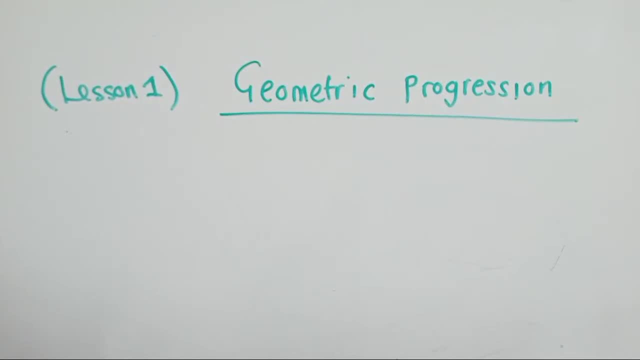 Yeah, just comment. if it's clear, We start. Okay, Susan, I can see Susan Banda is saying good evening, All right, So let me just start For those who have not yet joined. they will join us later, All right. So this is lesson one, And when it comes to this topic- geometric progression- this is a topic that 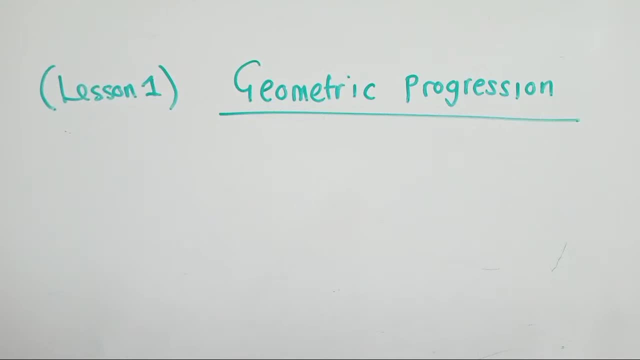 that quite number of people face difficulties on. The reason is they forget to follow simple rules. Okay, They forget to follow simple rules. So, rule number one: you must understand the terminologies, Terminologies, So you can get a paper. If you have a paper, you write what I'll be writing here. 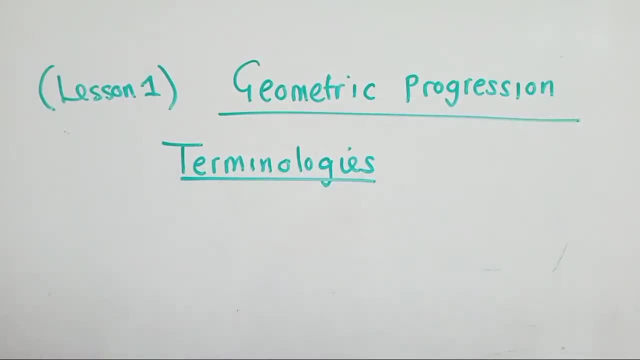 What are the terminologies? So there are basically a few terminologies that we must know. Okay, One of them is the first time, The one of the first time times. So when we say first time, This is denoted by always like a Okay. So what this first time is all about is the term to be used with the first time. 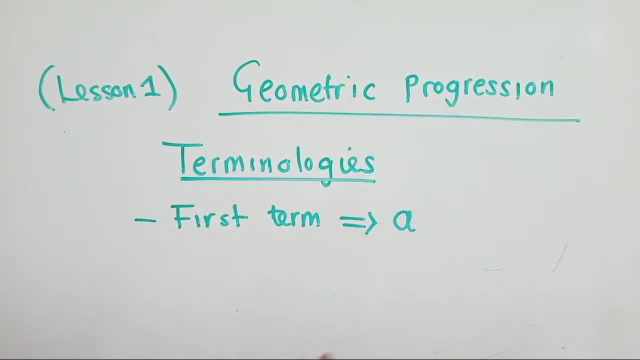 So me, prince nxy. I think it also says that you have to determine your first term. right is to know that the first term is going to take place somewhere else, not because you have to have a hope and your use all of her. 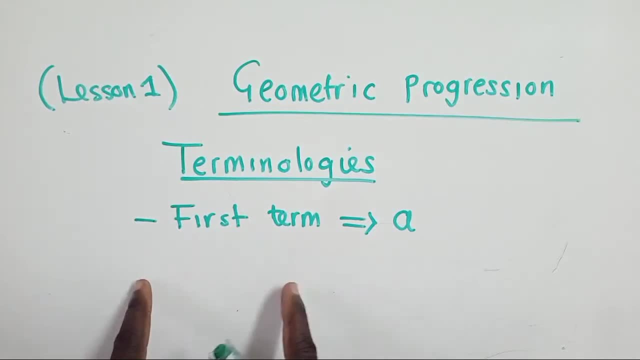 And once you know, I say the term I. now what I want to do is another ending and not test, because I've obviously fear. if there's a chance that you're already at is the number that is at the beginning or starting point of the sequence. okay. 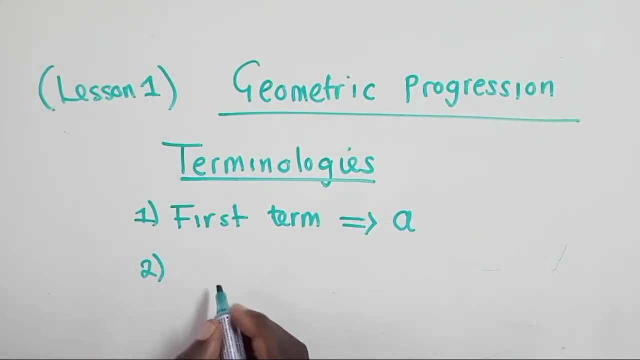 The next thing that we must be aware of is the common ratio. common ratio. This is also denoted by letter R After the common ratio. we must be aware of the position- It's also important- denoted by this nth, mostly n. I'll just say n, okay. 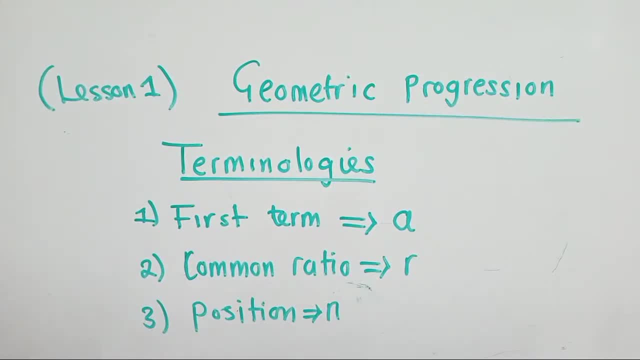 These things are very important. okay, When it comes to Geometric progression, All right. so, after knowing these terminologies, there is something else you must stick to, and these are formulas. Okay, The formulas. they are also very important. 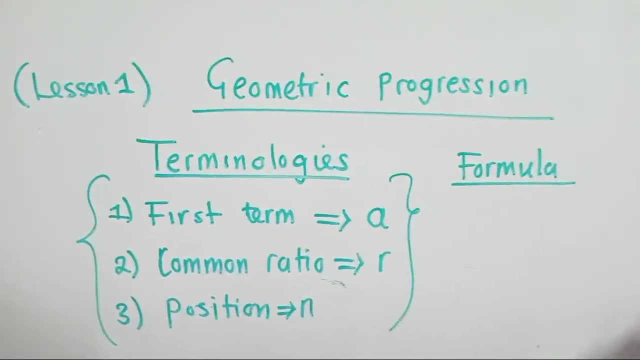 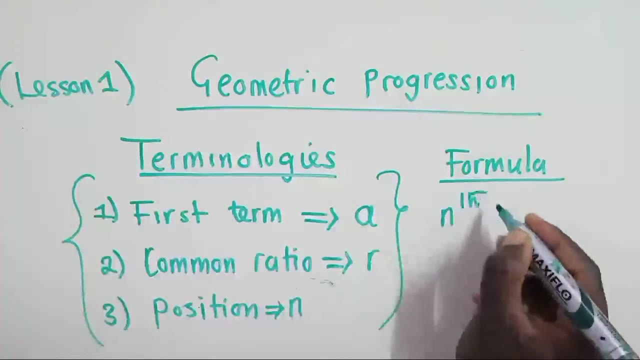 So the first formula, that's That you must keep in mind, is the nth formula, Formula for finding the term which is A multiplied by R power, n minus c, 1. This is important. This is formula number one. It's for the sum. 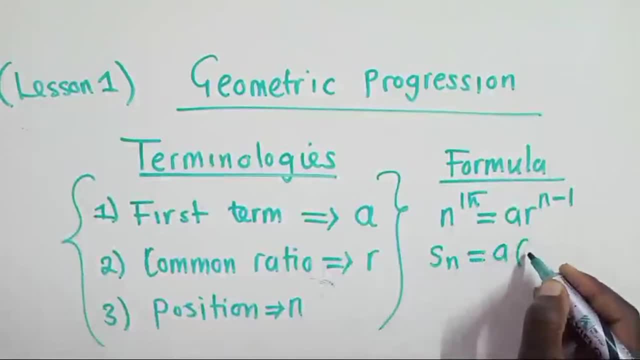 So these are the formulas. So keep on watching and at the end we'll try to do some examples. So this is the formula for finding the sum. okay, So formulas for finding sum. there are two of them. okay, We've got the one I've written here. 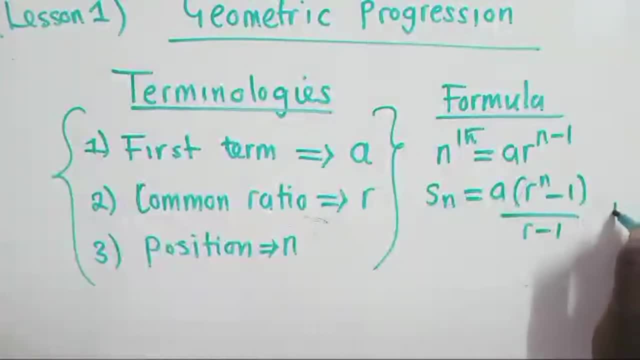 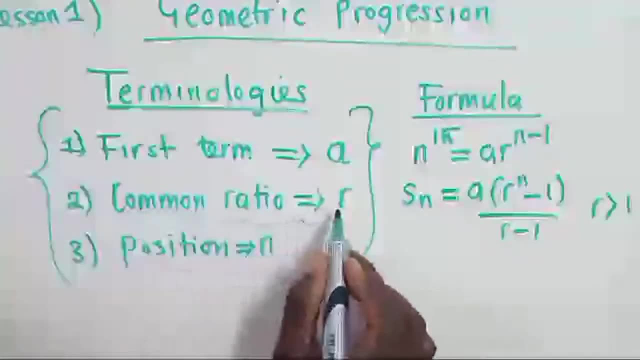 We use this one when R R, the R is greater than 1.. So when you find what we call common ratio, which is the R, you find that it's It's greater than 1.. Maybe you have a two of this formula. 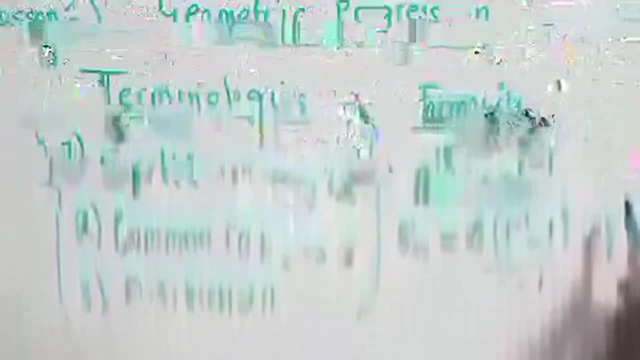 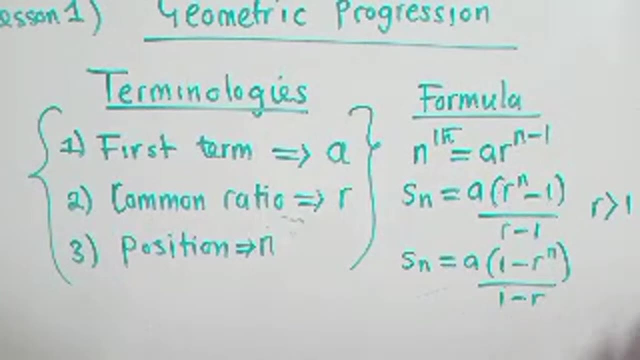 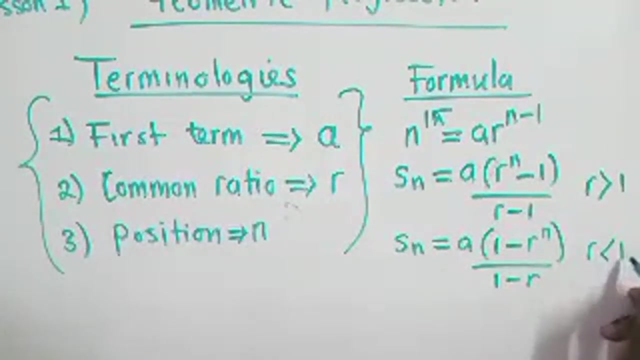 Another formula for finding sum. it's right here. It's almost the same, but you must switch the position of R, Like that. okay, So now this one. we use it when our R is less than 1, okay, Okay. 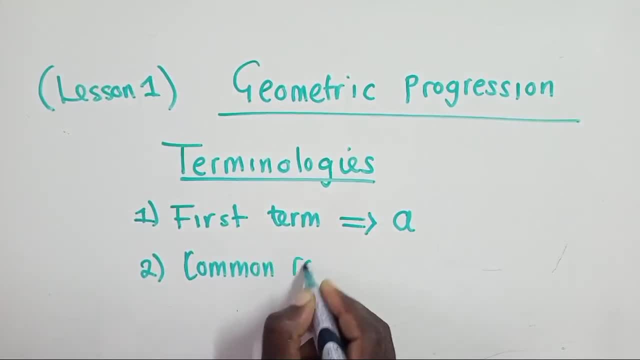 ratio. this is also denoted by letter r after the common ratio. we must be aware of the position. it's also important, denoted by this nth, mostly n. i'll just say n. okay, it's, these things are very important. okay, when it comes to geometric progression, all right. so, after knowing these terminologies, 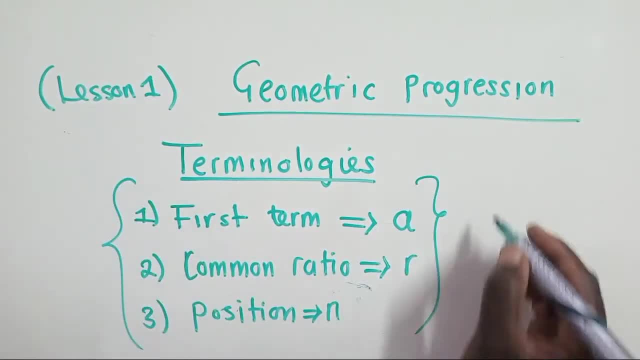 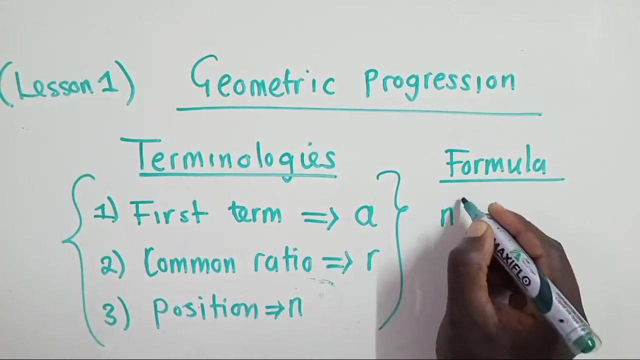 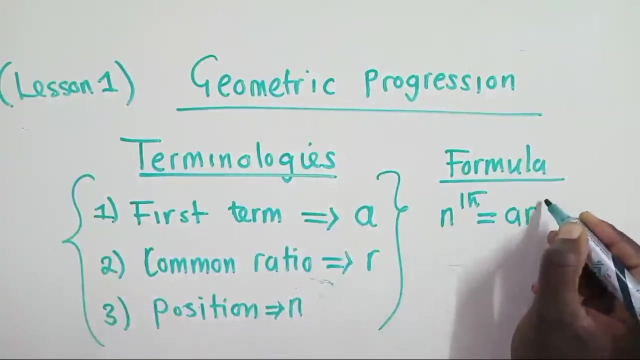 there is something else you must stick to, and these are formulas. okay, the formulas, they are also very important. so the first formula thus that you must keep in mind is the nth formula, formula for finding the term which is a multiplied by r power, n minus c one. this is important. this is formula number one. 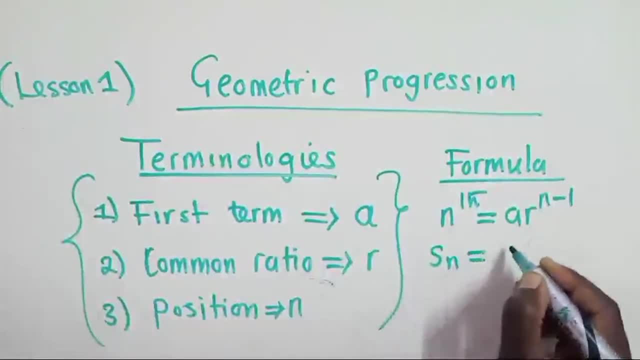 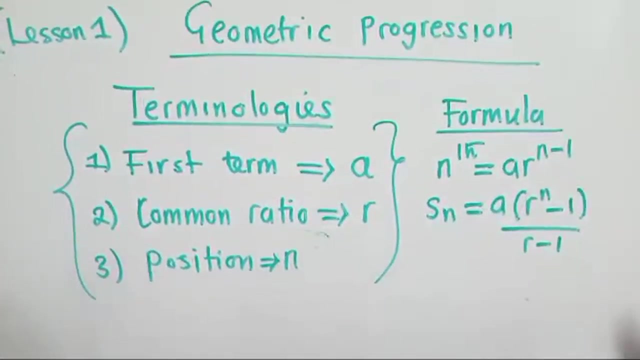 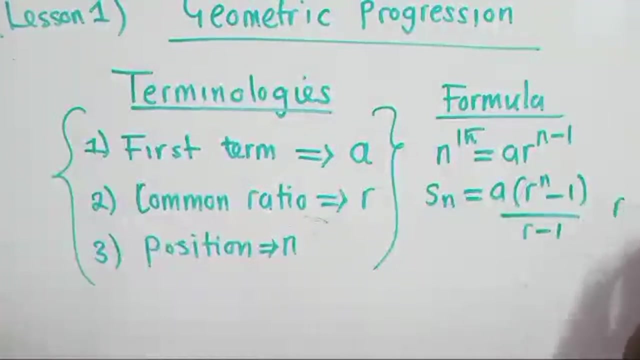 it's for the sum. so these are the formulas. is? this is the formula for finding the sum? okay, so formulas for finding some there. okay, we've got the one i've written here. we use this one when era air r, The r is greater than 1.. So when you find what we call common ratio, which is the r, 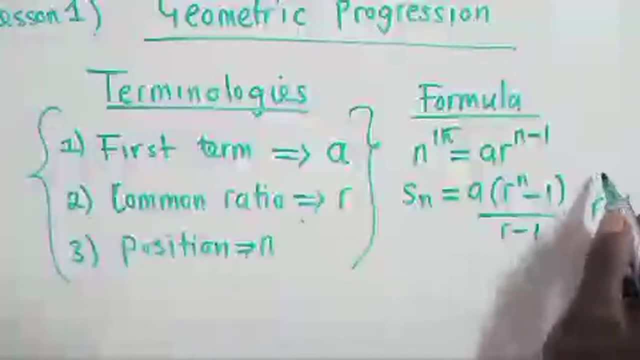 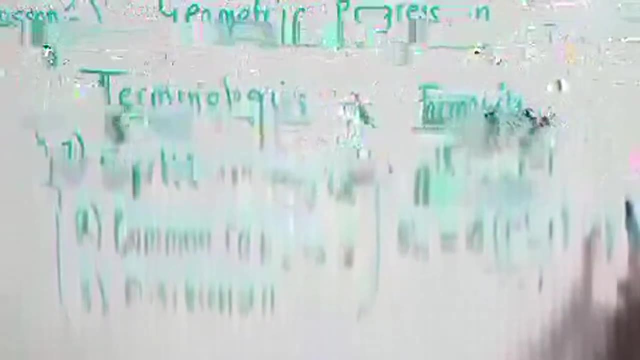 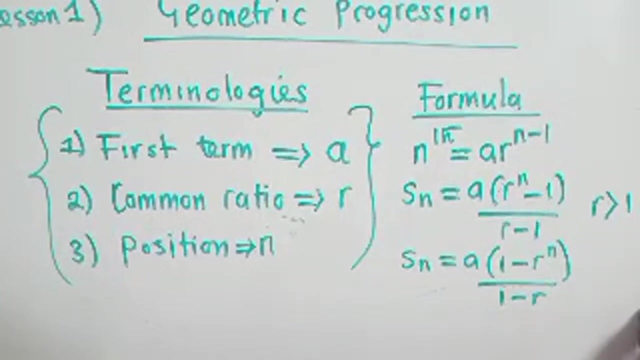 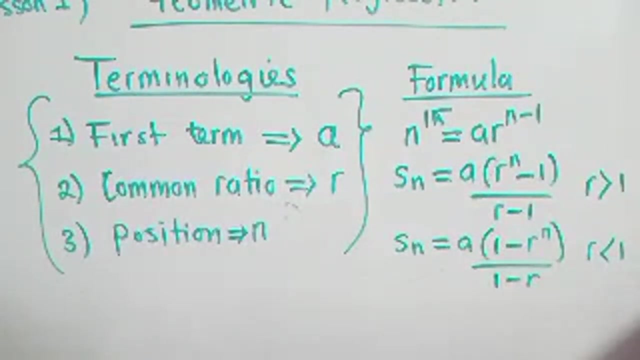 you find that it's greater than 1.. Maybe you have a 2 of this formula, Another formula for finding sum. it's right here, It's almost the same, but you just switch the position of r like that. okay, So now this one. we use it when our r is less than 1, okay. 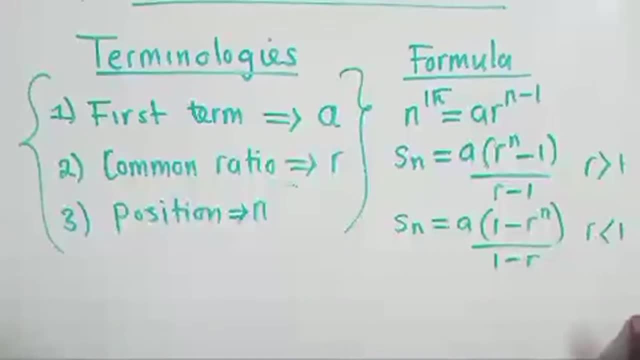 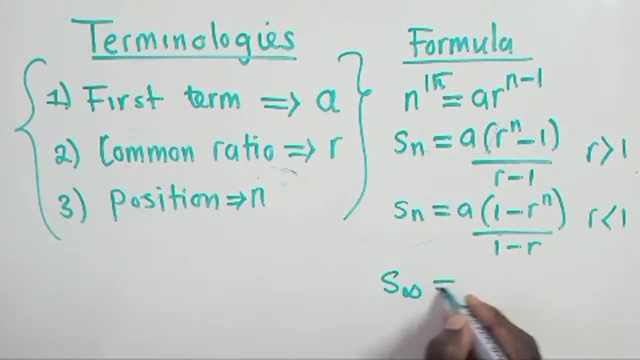 Okay, Another formula that you must be aware of is for finding sum to infinity. So, for sum to infinity, what is it? What is the formula for sum to infinity? If you're following, are you following To confirm if you're following? remember, at the end we'll do a little bit of some examples. 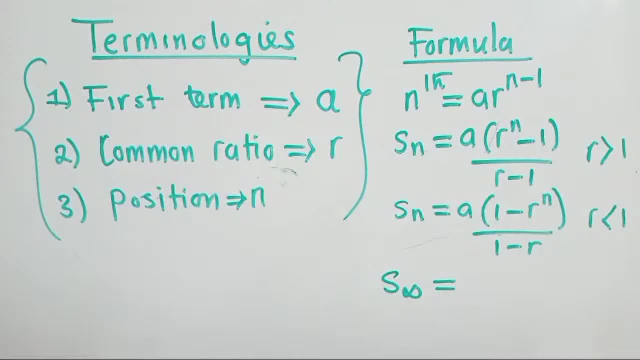 so that we know on how all these things work. okay, Are you there? So now, what is the formula for sum to infinity? The formula for sum to infinity will just look like this. okay, Very simple, just like this, Okay. 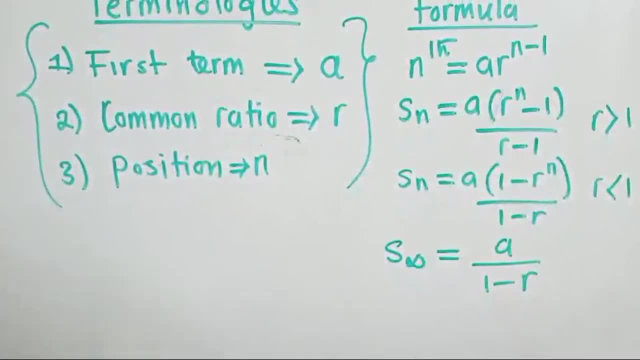 And last but not the least is the formula for mean. So just write gm geometric mean. So this is how the formula will look like. All right, So now let's try to jump into an example, since we've talked about the terminologies and the formulas to use here. 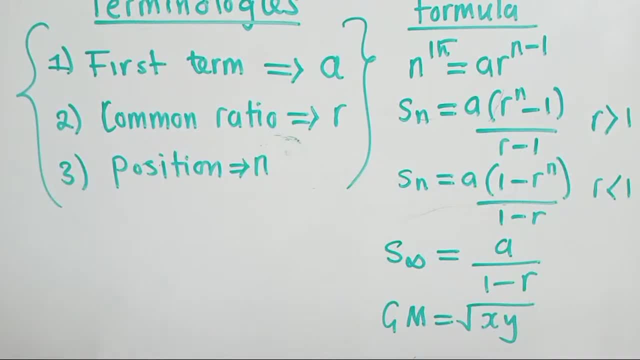 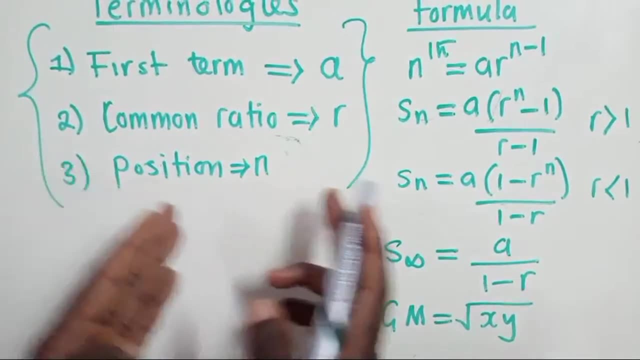 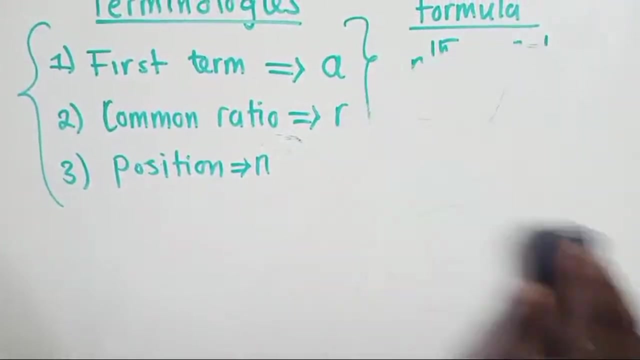 So let's look at the example, one example that we need to understand, on how to apply all these things that are here. okay, So let me copy or let me write an example for you. So, for this example, try to work it out, okay. 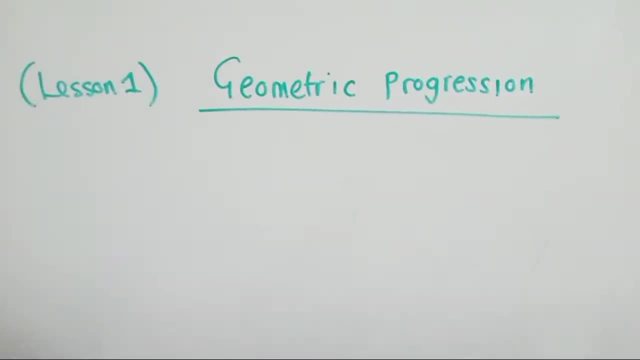 And this is lesson one. By the way, if you have just joined, this is lesson one. Keep on following my videos. time and time We'll be doing live like this, where we discuss a few things about the topic, So let's get started. 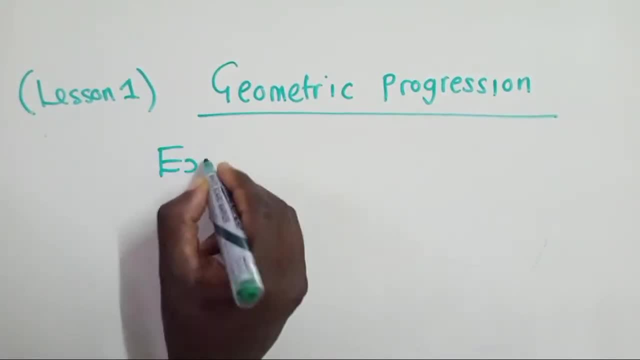 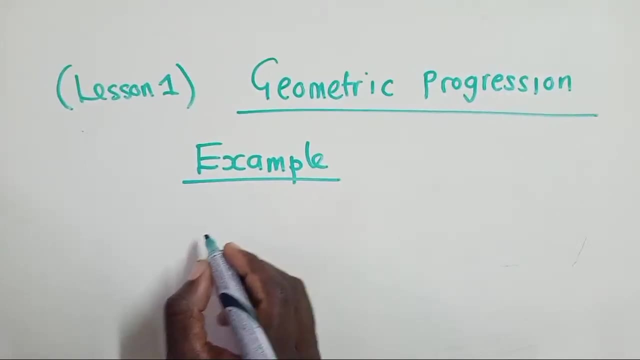 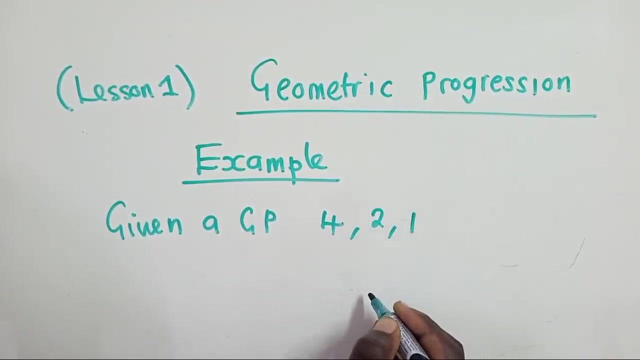 Thank you. So example: So start solving this example and see the answer that you get if we are going to get the same answer. So, given a g p, okay, That is 4, 2, 1.. Okay, 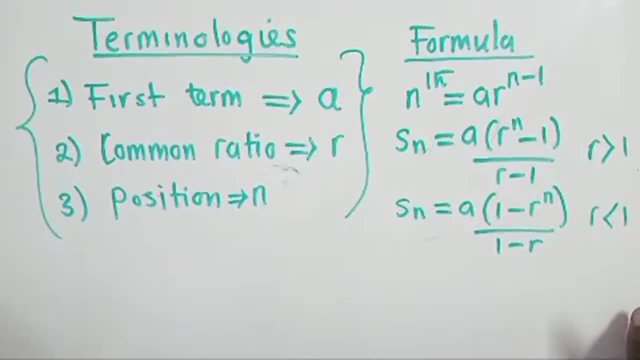 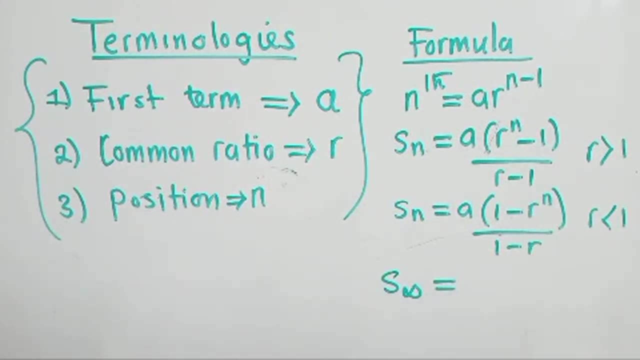 Another formula that you must be aware of is for finding sum to infinity. So, for sum to infinity, what is the formula for sum to infinity? If you're following, are you following To confirm if you're following, remember at the end we'll do a little bit. 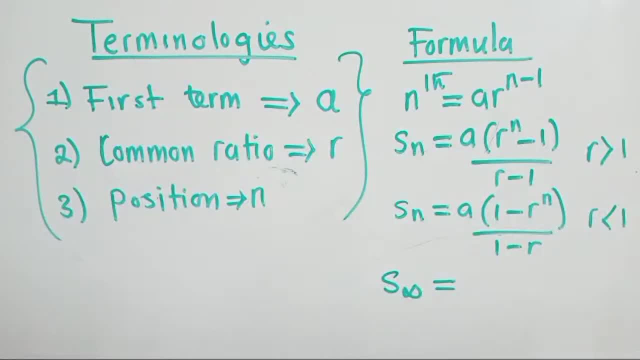 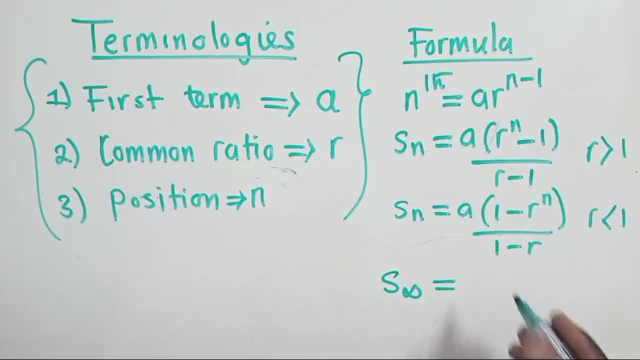 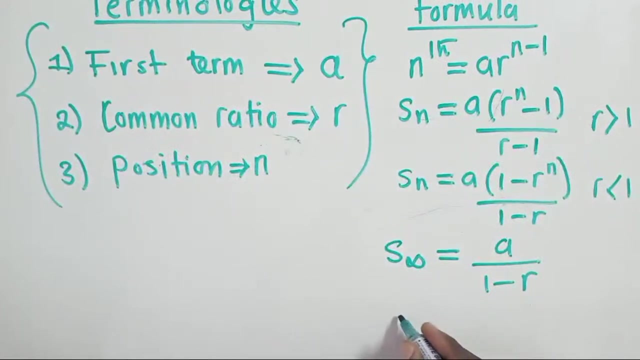 Okay, Okay, Okay, Okay, Okay, Okay. So now, what is the formula for sum to infinity? The formula for sum to infinity will just look like this. okay, Very simple, just like this. And, last but not the least, is the formula for mean. 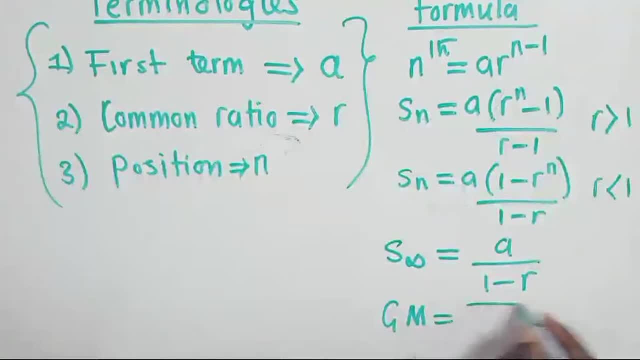 So just write GM: geometric mean. So this is how the formula will look like. All right, So now let's try to jump into R. So let's try to jump into an example, since we've talked about the terminologies and the 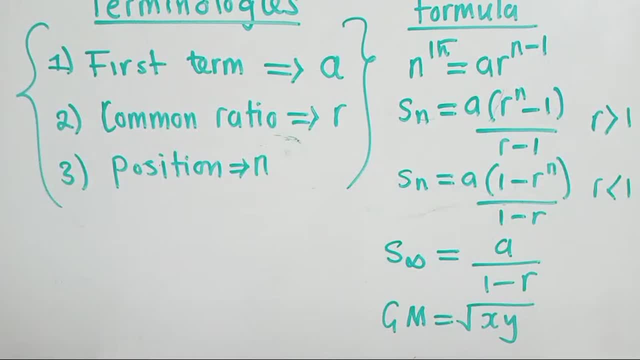 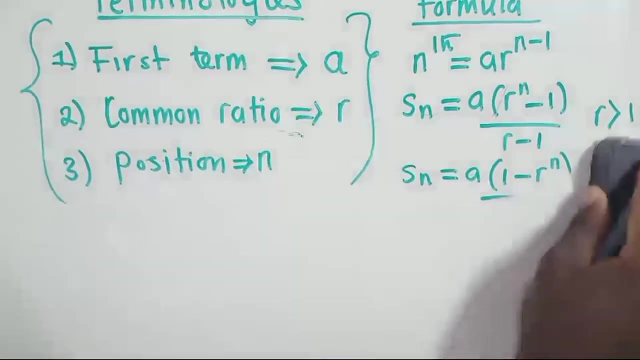 formulas to use here. So let's look at the example, one example that we need to understand on how to apply all these things that are here. okay, So let me copy or let me write an example for you. So, for this example, try to work it out, okay. 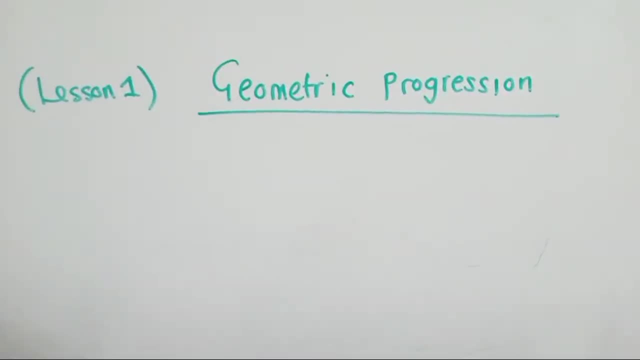 And this is lesson one. By the way, if you have just joined, this is lesson one. Keep on following my videos. time and time We'll be doing live like this, where we discuss a few things about the topic that we pick. 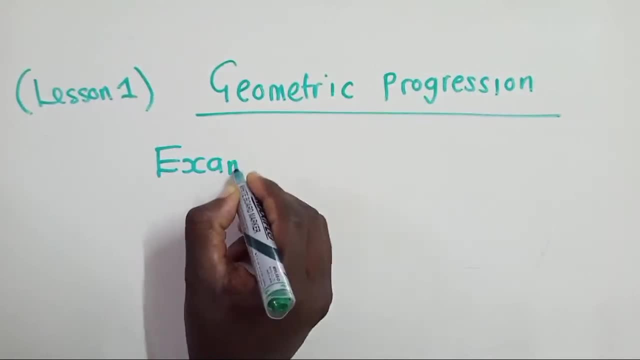 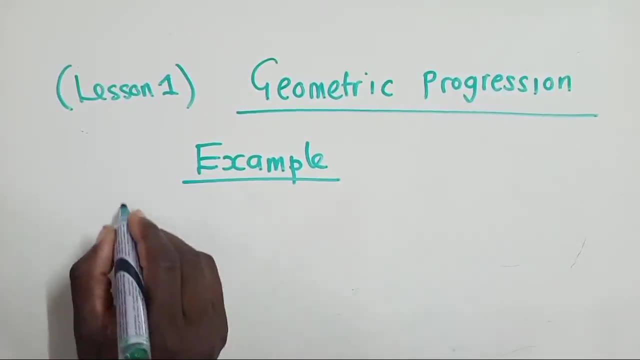 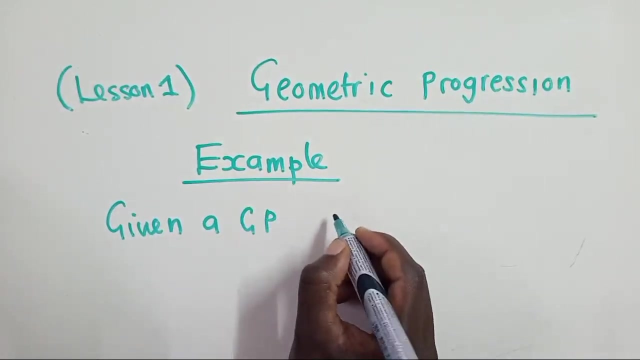 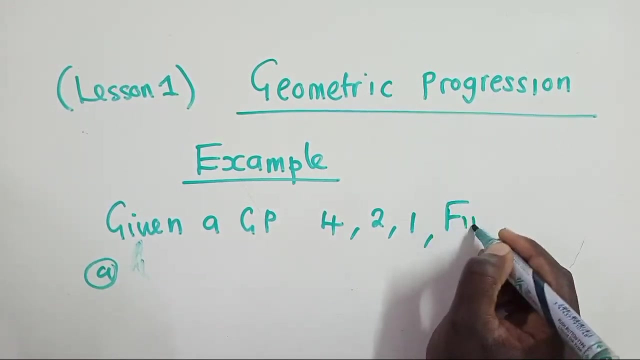 So example: So start solving this example and see the answer that you get, if we are going to get the same answer. So, given A GP, Okay, that is a four comma, two comma one. Okay, A find find A the fifth term. 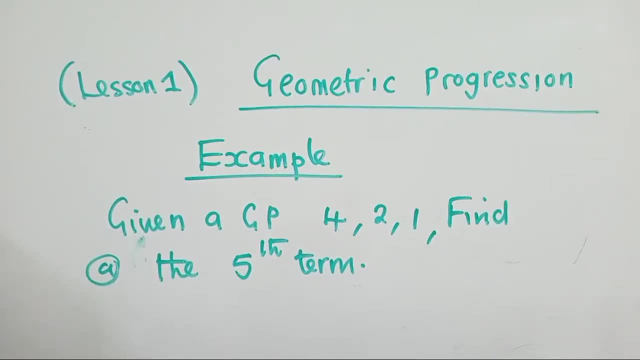 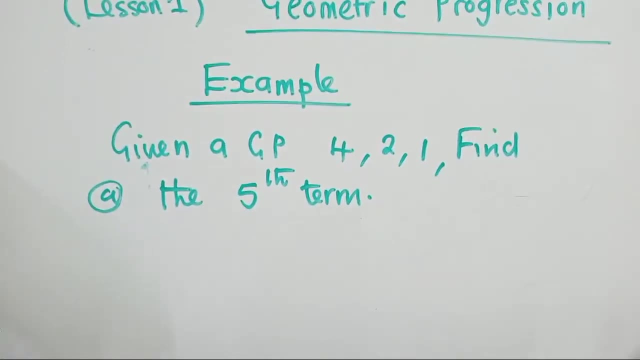 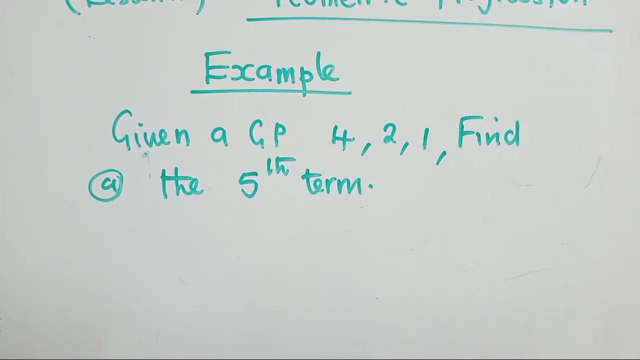 So this is A. I've got about three questions. So this is A. we need to find the fifth term. So how do we find the fifth term? The first thing that should come in our mind is the terminologies. So under the terminologies, we know that of course there must be A, there must be N, there must be R. 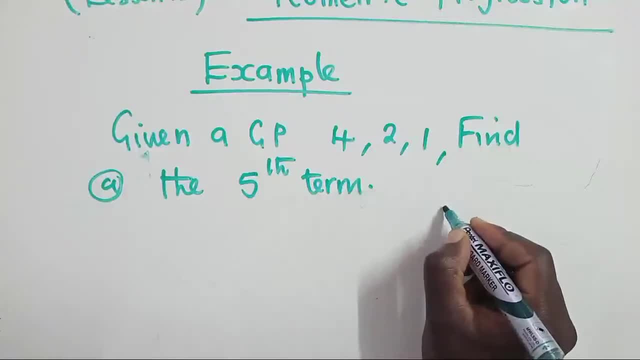 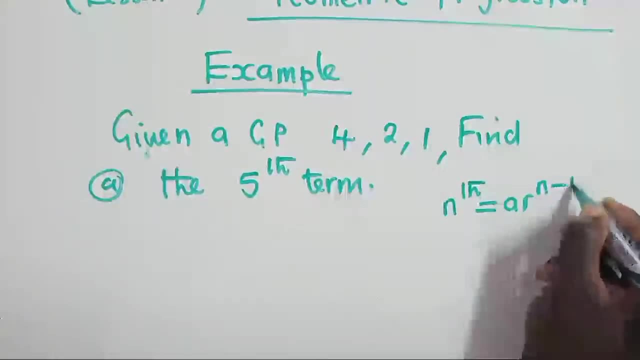 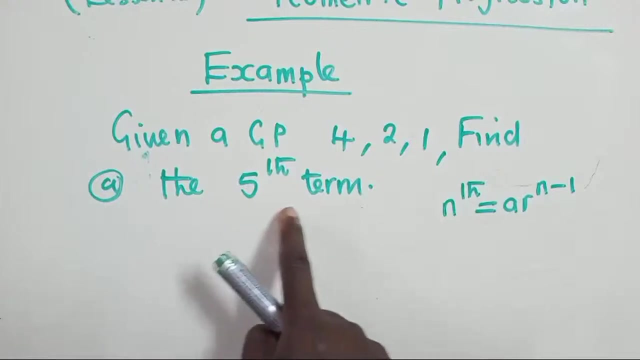 Okay, so what formula are we going to use? It's for the term, So we shall say: N is equal to A R power N minus. Okay, so this is the formula, one of the formulas that we need to use. This formula is specifically for finding the term. 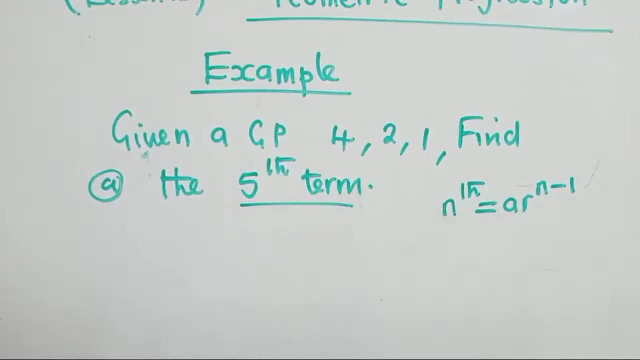 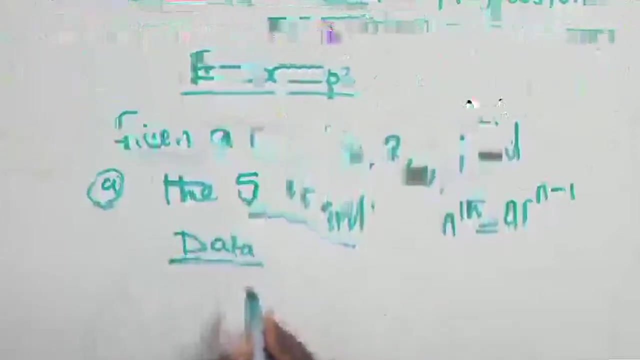 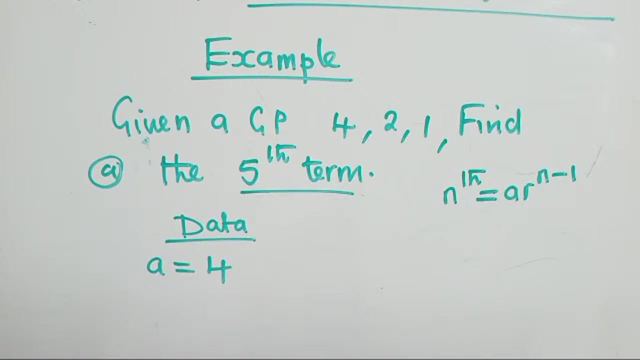 Whenever you see term, just know that you're dealing with this formula, the word term. So let's gather our data. Very important: What is our A? What is Our A? our A is a four. Remember I said the term, the number that is at the starting point of the sequence. 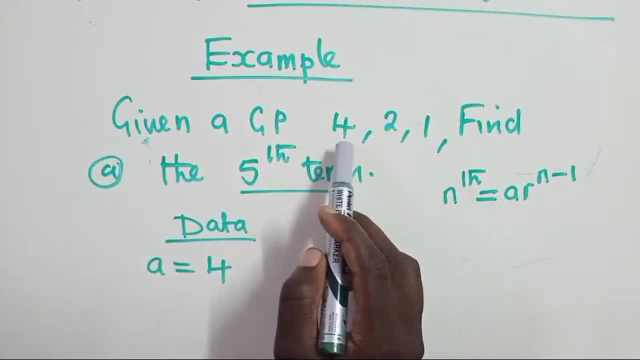 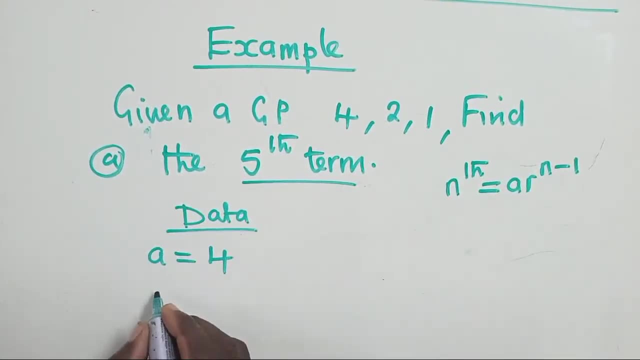 Look at this sequence: the number that is a starting at the starting point is a four. Okay, So once you write that, you now go to the N. What is our N? It's a position. Mostly it's what you've been asked. 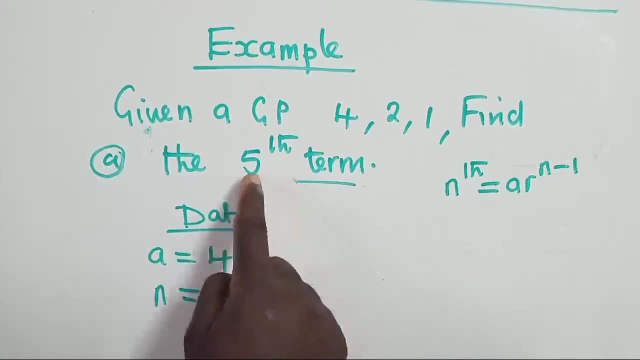 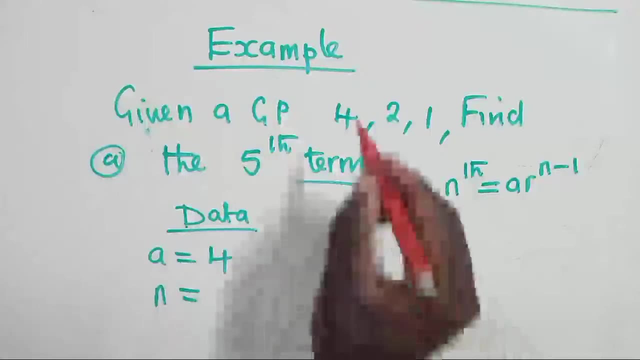 In the question they have asked us to find the fifth, this five. So we're trying to find the number that is at position five. Look at this: At position one- this is, of course, the first term- We have a four. 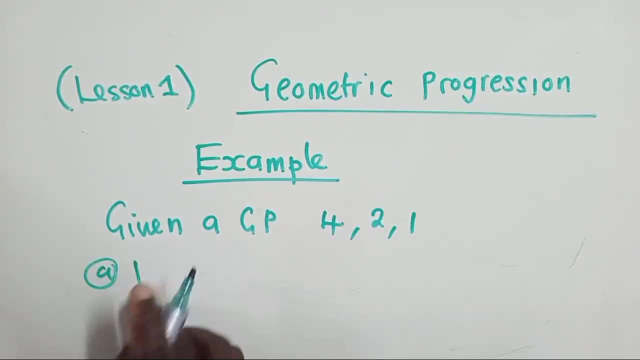 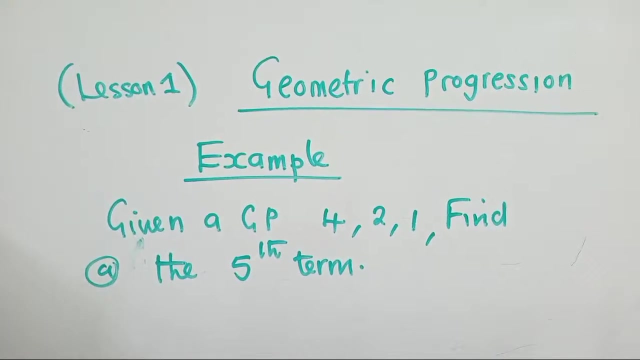 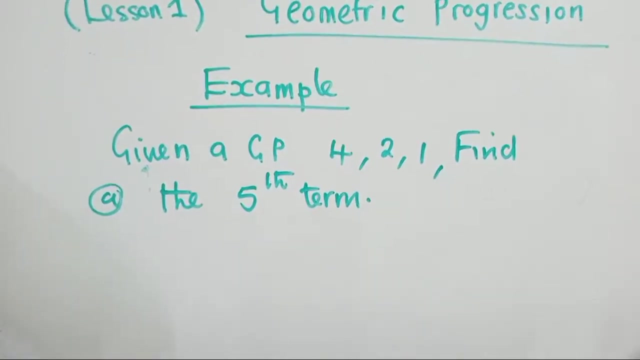 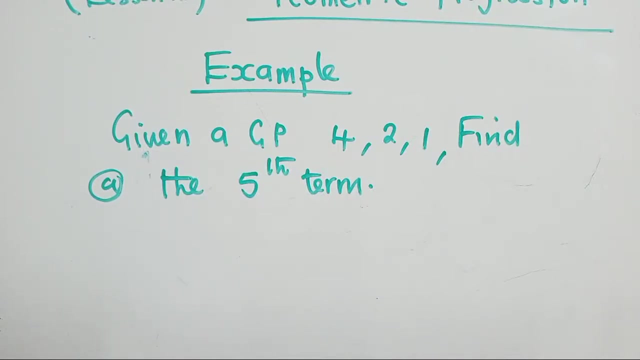 A, Find, Find, find, a the fifth term. So this is a. I've got about three questions, So this is a. we need to find the fifth term. So how do we find the fifth term? So the first thing that should come in our mind is the terminologies. 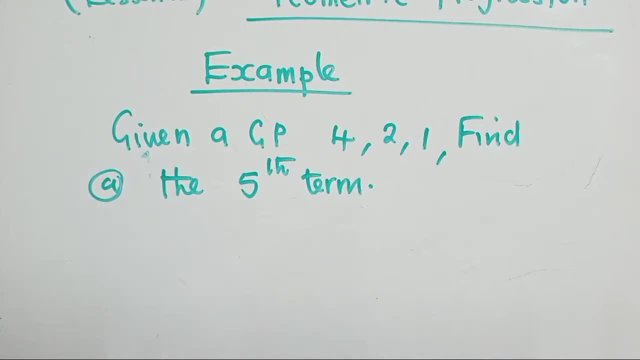 So, under the terminologies, we know that of course there must be a, there must be n, there must be r. Okay, So what formula are we going to use? It's for the term. So we shall say: n is equal to a, r, power n minus. 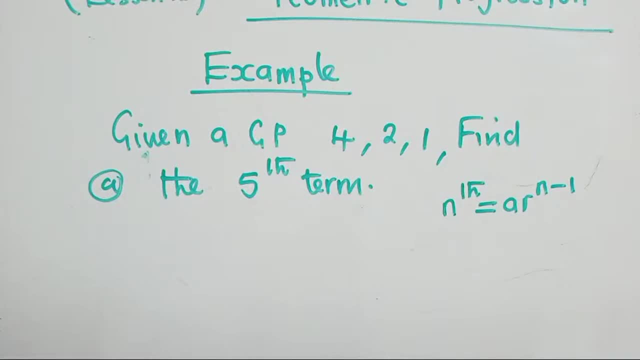 Okay, So this is the formula, one of the formulas that we need to use. This formula is specifically for finding the term. Whenever you see term, just know that you're dealing with this formula, the word term. So let's gather our data. 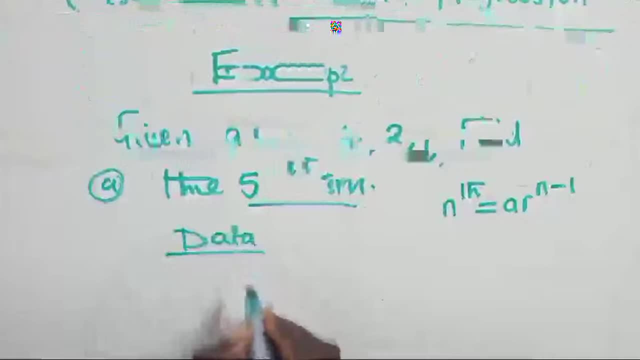 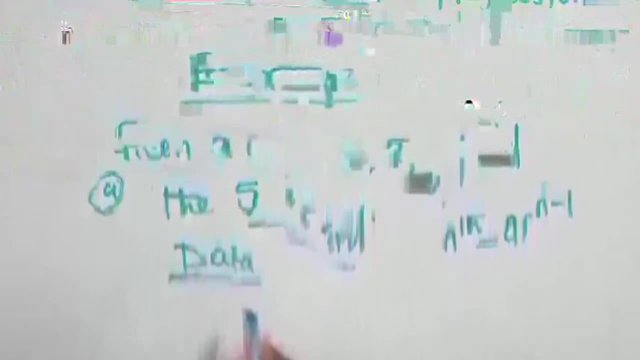 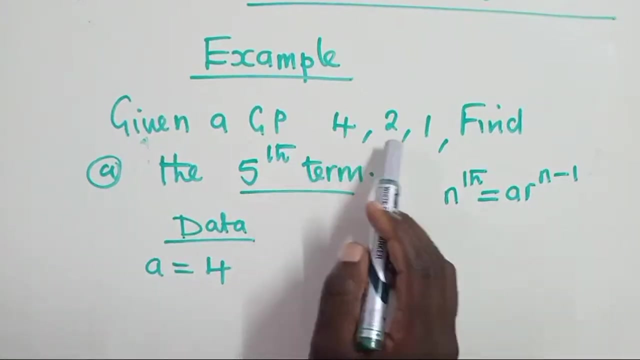 Very important. What is our a? What is our a? Our a is a four. Remember, I said the term, the number, The number that is at the starting point of the sequence. look at this sequence: the number that is a starting, at the starting point, is a four. okay, 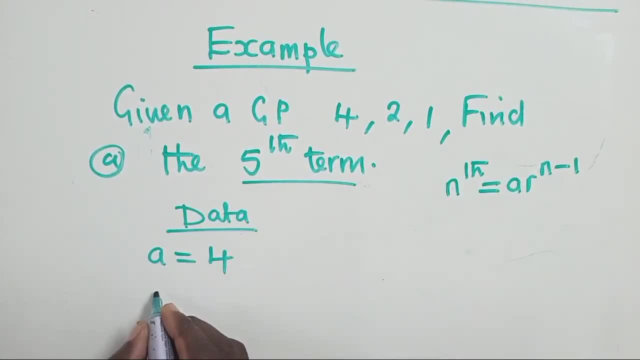 So once you write that, you now go to the n. what is our n? It's a position. Mostly it's what you've been asked in the question. They have asked us to find the fifth, this five, so we are trying to find the number. 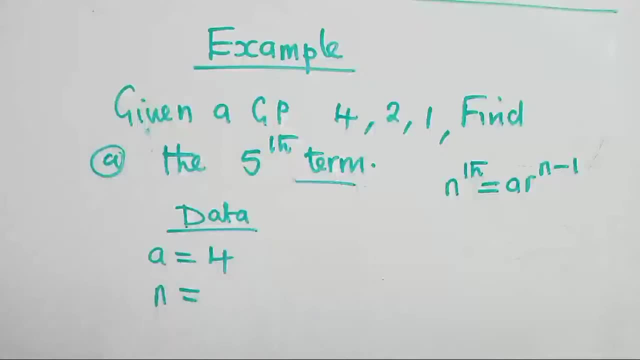 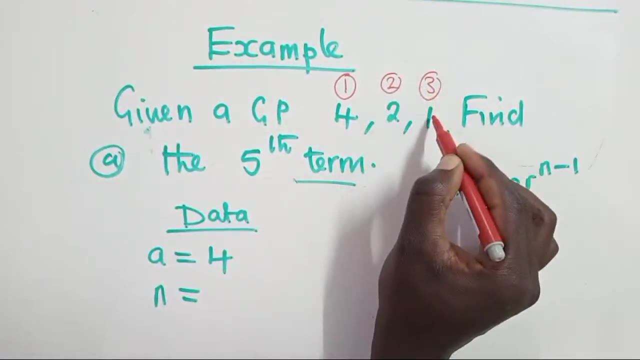 that is at point n. So we can now find the fifth at position five. Look at this. At position one- this is of course the first term- We have the four. Position two: we have the two. Position three: there is a one. 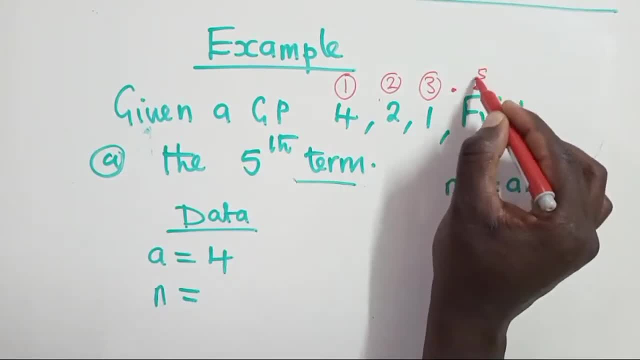 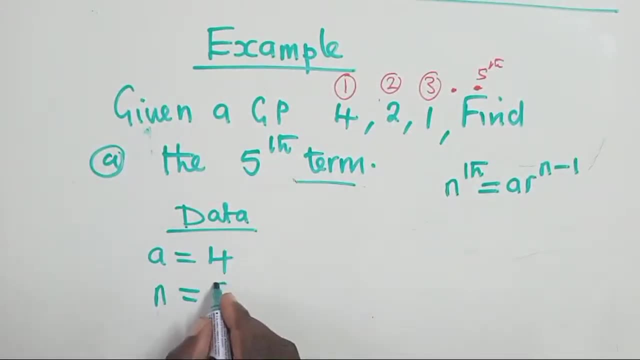 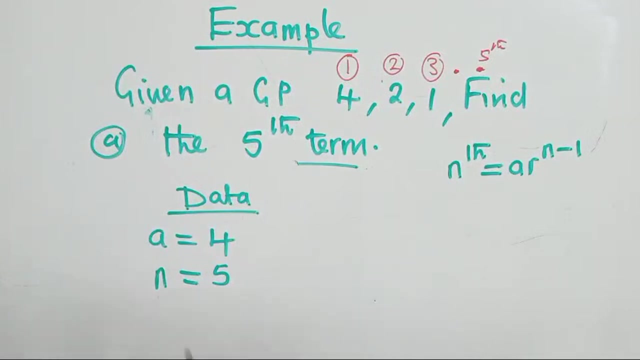 Position four? we don't know. Position five is what we've been asked to find. Position five. So we shall say fifth is what we are looking for. So it's a five. We write our five there. So after writing that five hours we can now find the fifth. 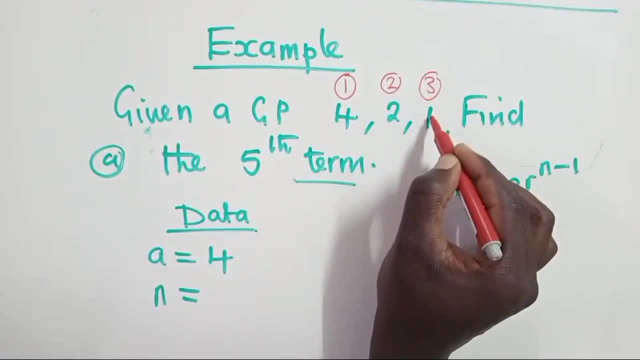 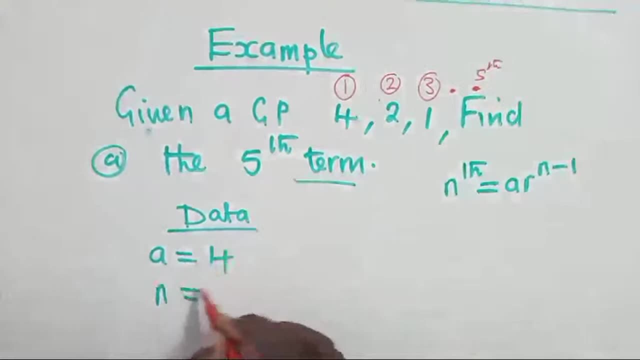 Position two, we have a two. Position three, there is a one Position four, we don't know. Position five is what we've been asked to find, Position five, So we shall say fifth is what we are looking for. So it's a five. 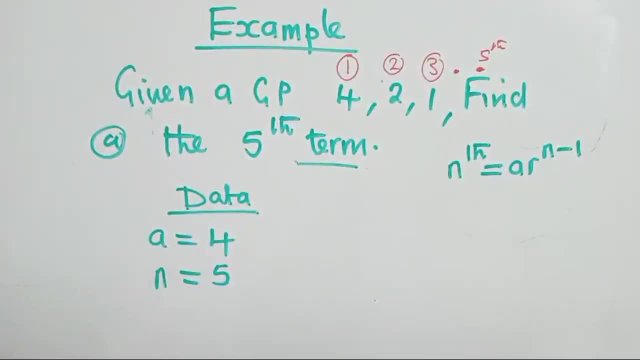 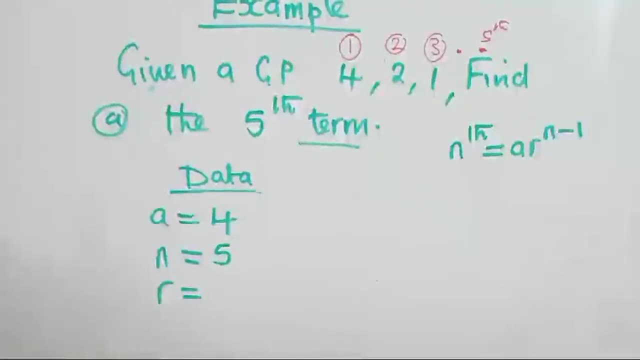 We'll write our five there. So after writing that five words, we can now find our R. What is our R? So our R is: either you write 1 over 2 or 0.5.. So whichever you think is easier working with a decimal number. 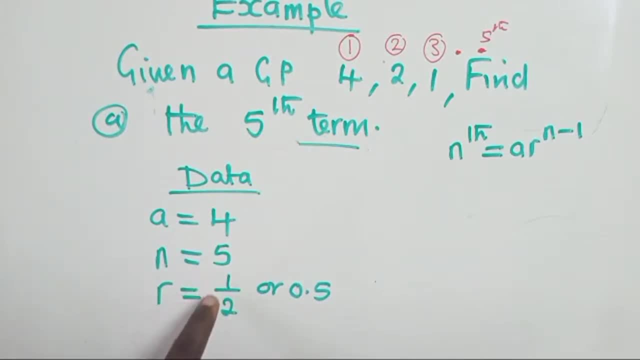 because these two things are just the same. So if you want, you can get 1 over 2 or 0.5.. So if you want, you can get 1 over 2 or 0.5.. 0.5. Whatever you think you're comfortable working with, it's okay. So I'll go with 0.5. 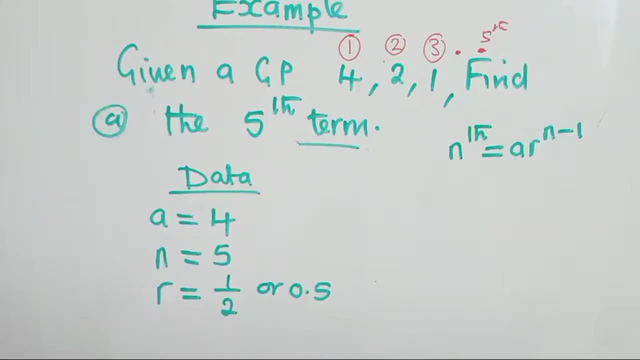 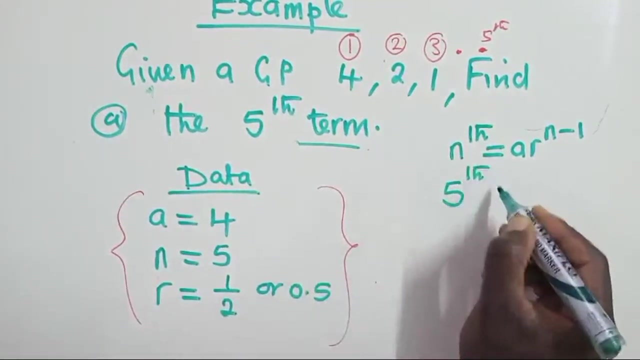 This is what most people like using, So I'll go with 0.5.. Upon gathering our data here, we can now plug them in the formula. So what are we looking for? On n, it's a five. that will be there. On a, there will be four. On r, there will be a 0.5.. On n: there we know it's a five minus. 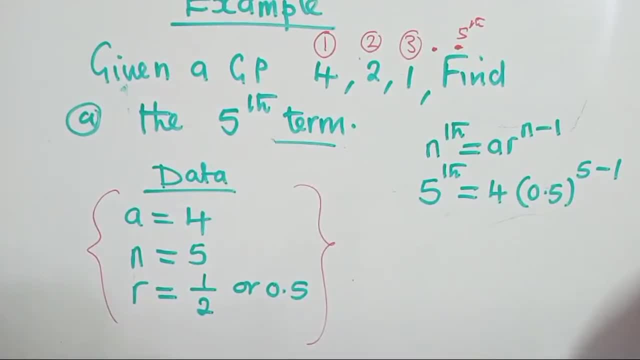 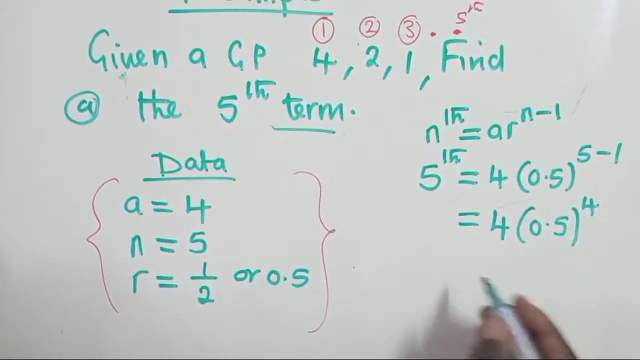 a one. Okay. So after doing this, you simplify. Now we'll be four. There, we have a 0.5, and we have a four. Okay, Because five minus one is a four. All right, So next. 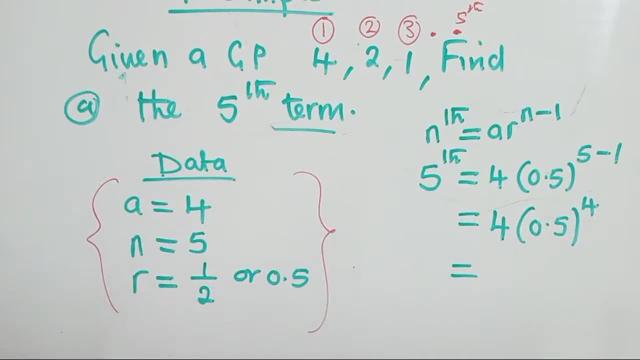 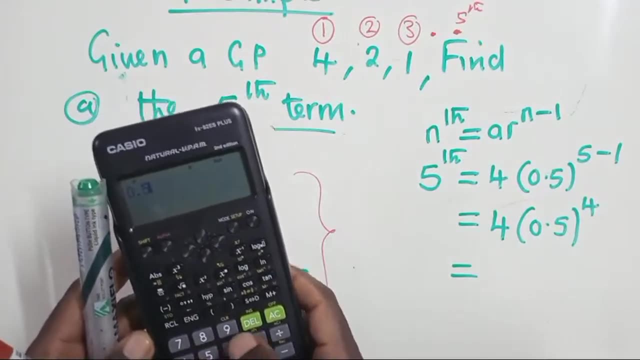 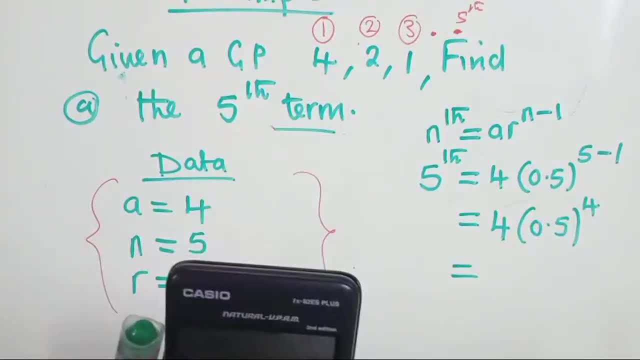 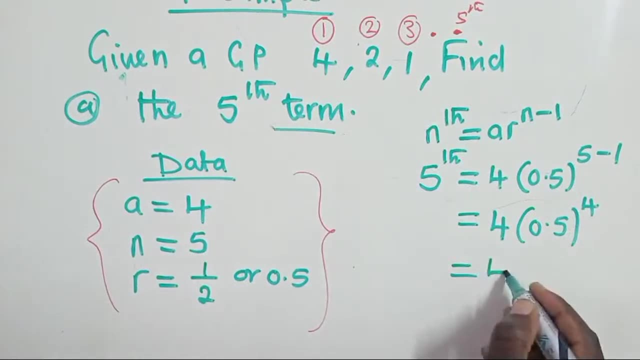 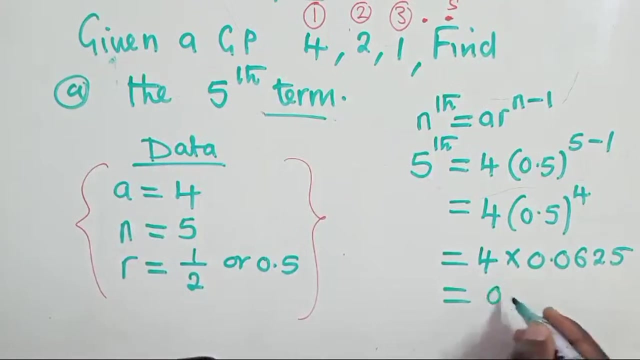 4.. So it will be 0, okay. So first let me start with the 4.. 4 times 0.0625,, okay. And when we multiply there, what is our final answer? It's, of course, 0.25.. So this is our. 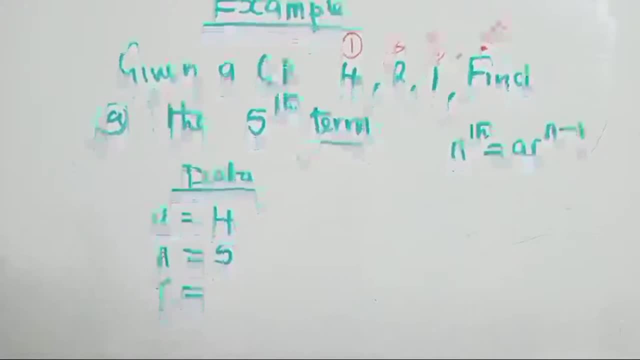 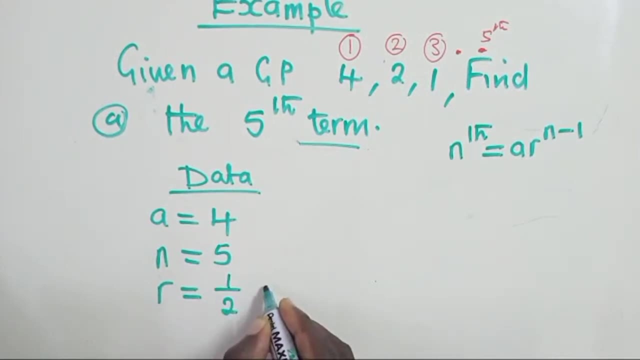 Okay, So let's give this one an answer: our R. What is our R? So our R is: either you write 1 over 2 or 0.5.. So whichever you think is easier working with a decimal number, because these two things are just the same. So if 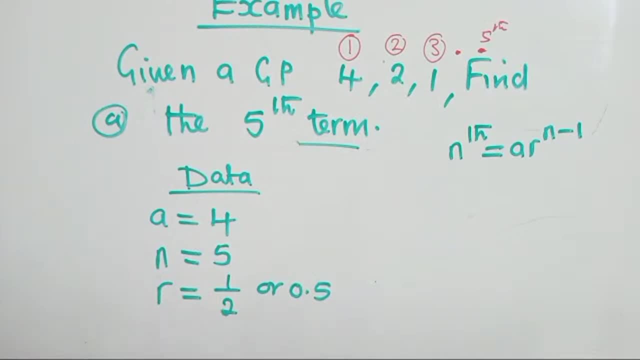 you want. you can get 1 over 2 or 0.5.. Whatever you think you're comfortable working with, it's okay, So I'll go with 0.5.. This is what most people like using, So I'll go with 0.5. 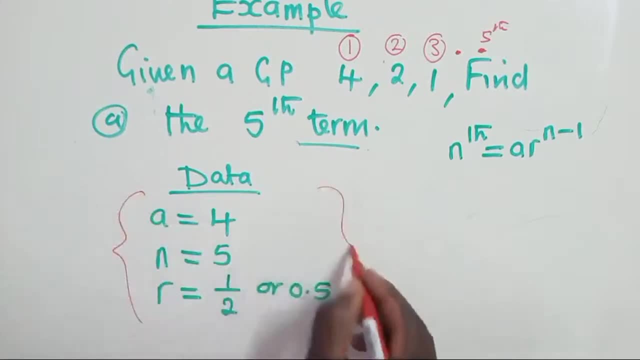 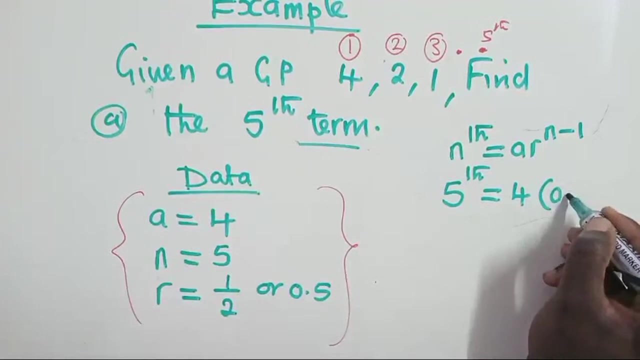 Upon gathering our data here, we can now plug them in the formula. So what are we looking for? On N, it's a 5, that will be there. On A, there will be 4.. On R, there will be a 0.5.. 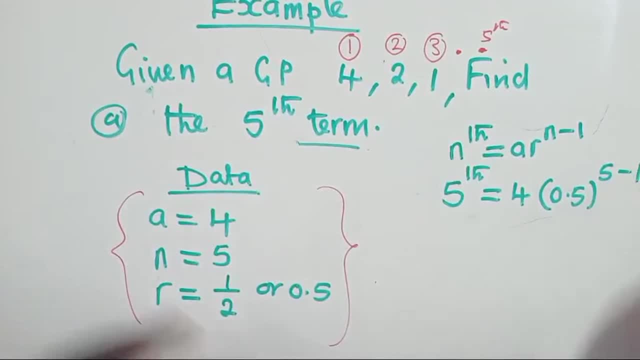 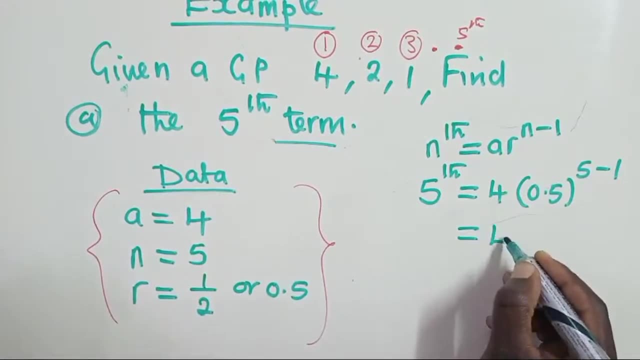 On N. there we know it's a 5 minus a 1.. Okay, So after doing this, you simplify now with the 4.. There we have a 0.5 and we have a 4.. Okay, Because 5 minus 1 is a 4.. All right. 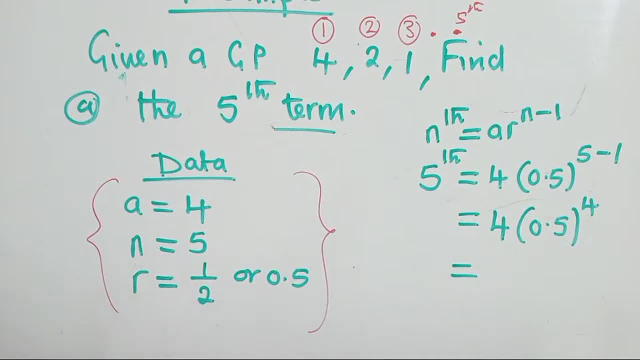 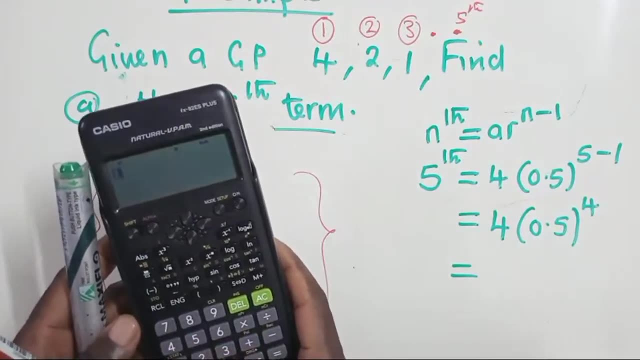 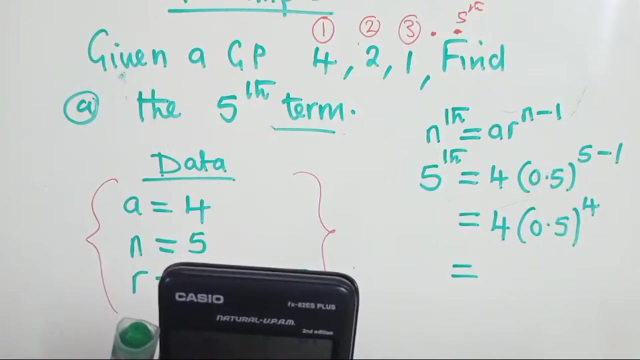 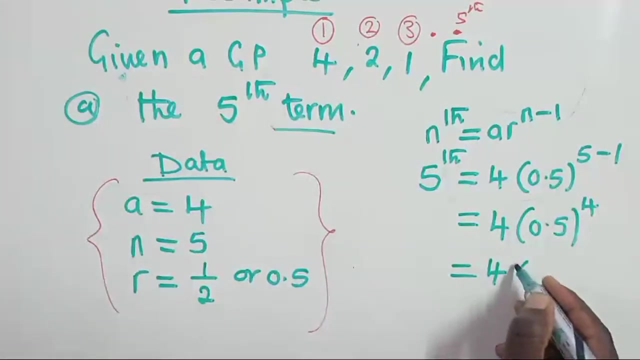 So next you just get your calculator- whichever calculator you're working with- you just say, uh, 0.5 power 4.. So it will be 0, okay. So first let me start with the 4. 4 times 0.0625, okay. 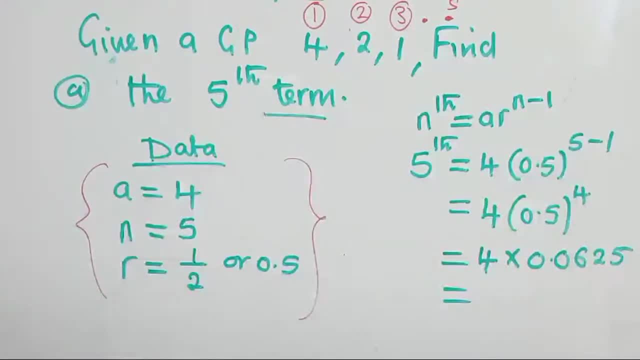 And when we multiply there, what is our final answer? It's, of course, 0.25.. So this is our final answer, Thank you. Thank you so much for watching Lesson 1.. Please make a date with me tomorrow, as I will be looking at the continuation of this. 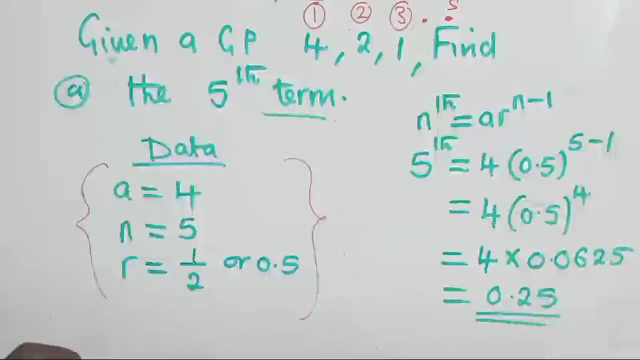 We'll call that as Lesson 2.. So, time and time, keep on joining me. I will be posting or I will be updating you on my Facebook page, as well as on my YouTube YouTube channel. if all the days that I'll be going live like this, 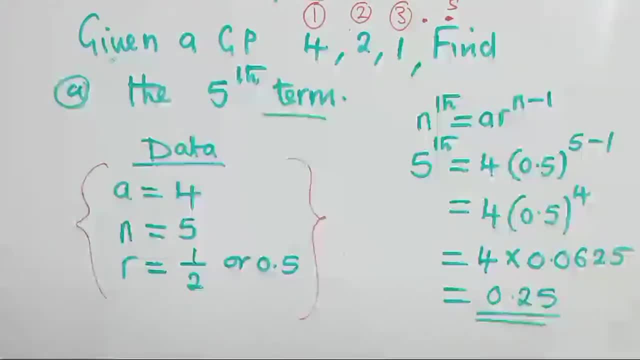 final answer, Thank you. Thank you so much for watching lesson one. Please make a date with me tomorrow, as I will be looking at the continuation of this. We'll call that as lesson two. So, time and time, keep on joining me. I'll be posting or I'll be. 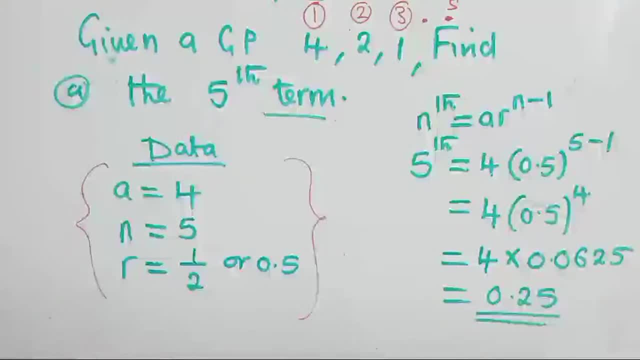 updating you on my Facebook page as well as on my YouTube channel, if all the days that I'll be going live like this, so that we keep on learning mathematics together, topic by topic. And to those who are asking: when am I going to do trig, we'll do trig after we finish this topic. 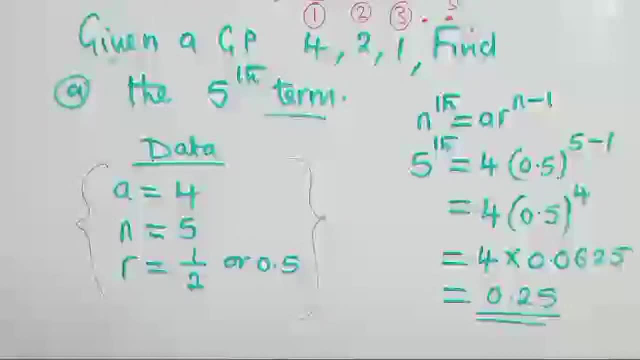 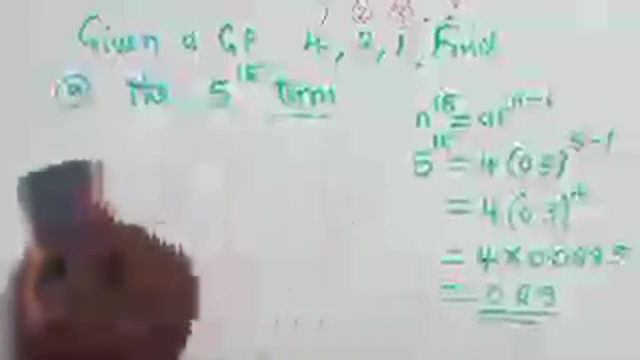 When we finish this topic. So that's a thing, And in case you're one of the people, as I keep on reminding you, I would like to join a WhatsApp group. As I can see there, Taita Stembo is asking about the WhatsApp group. We've got the WhatsApp group and classes. 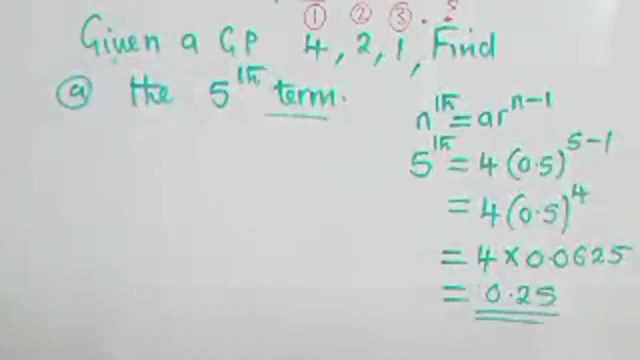 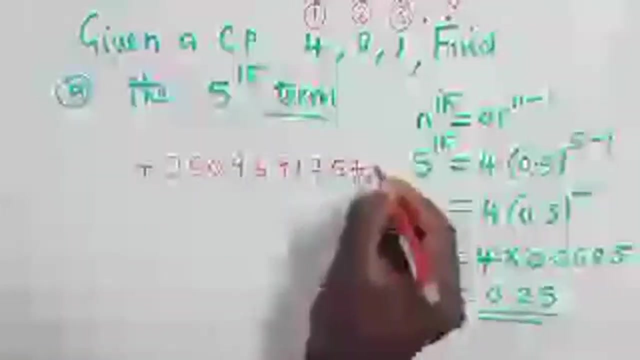 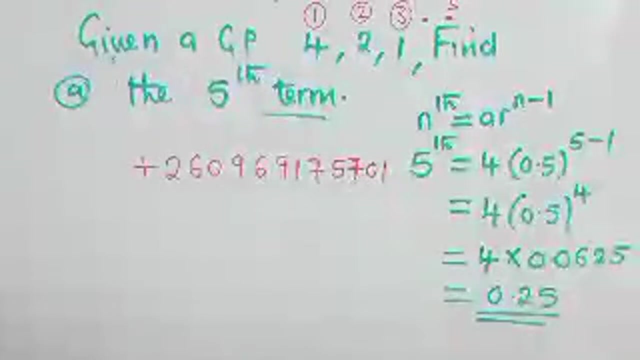 They always start at 20 o'clock Central African time. okay, So if you want to be part of that class, you of course can WhatsApp me on this number or call me on the phone. Or you WhatsApp or call and inquire what you need to do in order for you to be part of the class. Thank you and bye-bye.